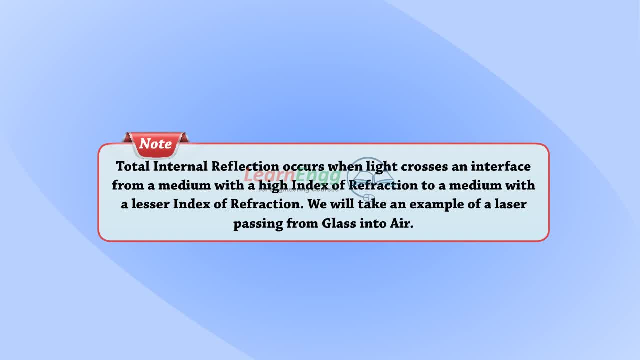 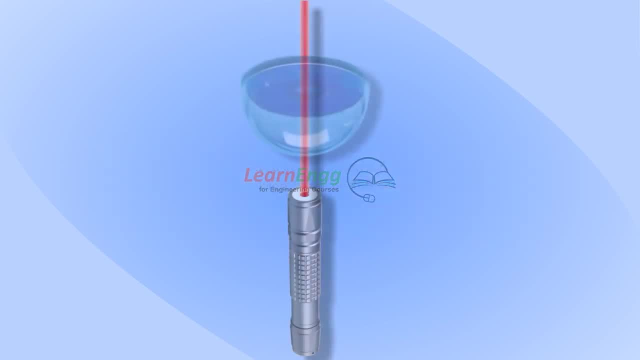 high index of refraction to a medium with a lesser index of refraction. We will take an example of a laser passing from glass into air, that is, from more denser to a low-denser medium. Then the light is refracted or bent toward the normal. 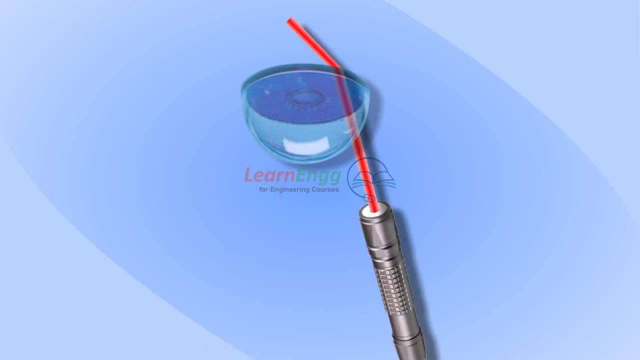 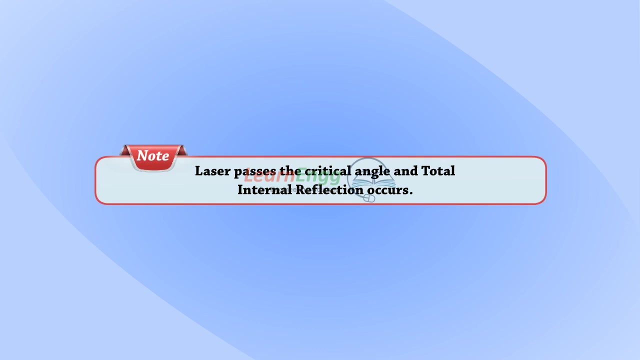 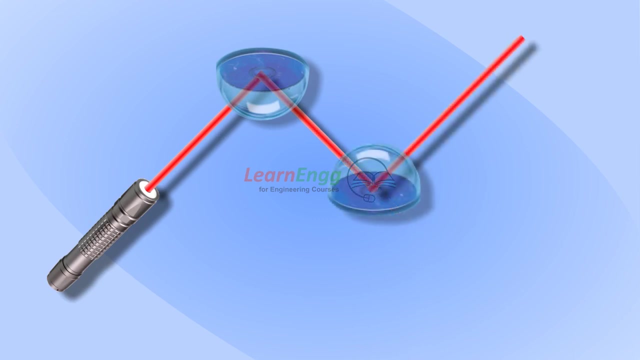 Light is also reflected. when light is reflected from a low-denser medium, Light is then reflected, Laser passes the critical angle and total internal reflection occurs. The critical angle is the angle of incident in an optical denser medium for which the angle of refraction is 90 degrees. 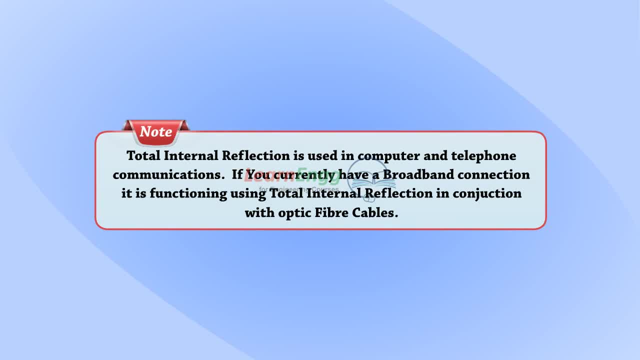 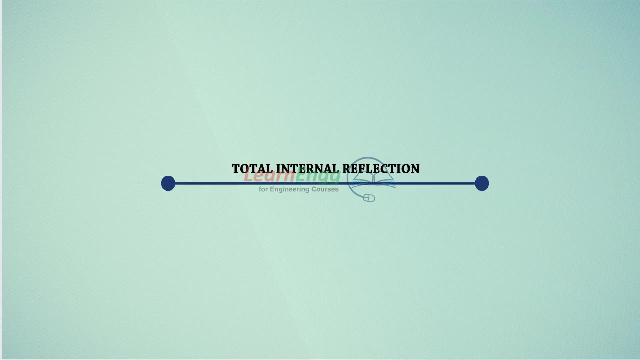 Total internal reflection is used in computer and telephone communications. If you currently have a broadband connection, it is functioning using total internal reflection in conjunction with optic fiber cables. In this video we are going to study about Total Internal Reflection. Light waves have three primary properties. that reflects total internal reflection. 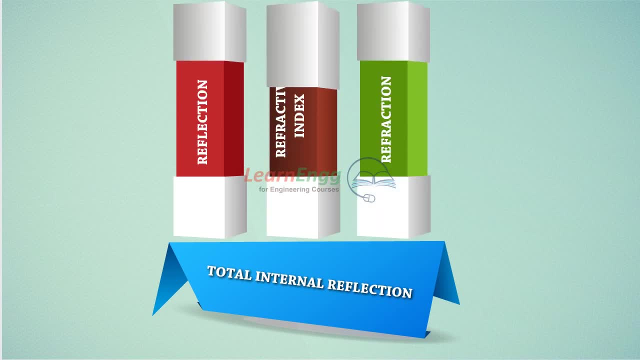 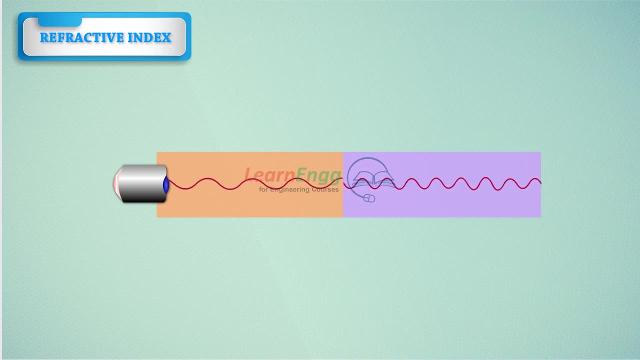 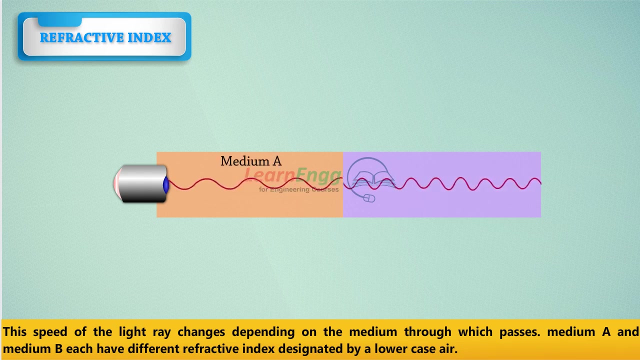 These are reflection, refraction and refractive index. We will see a light ray has propagates straight through two different mediums. This speed of the light ray changes depending on the medium through which passes. Medium A and medium B each have different refractive index, designated by a lower. 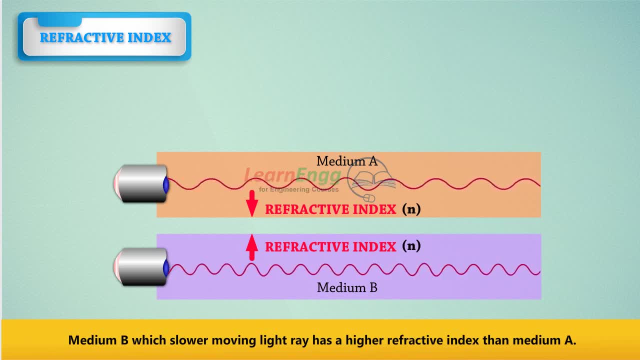 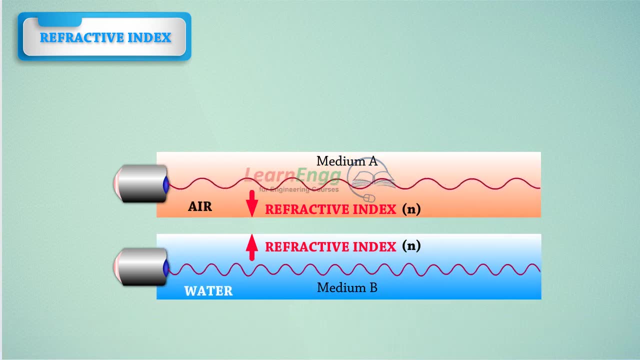 key than case n. Medium B with slower moving light ray has a higher refractive index than medium A. Medium B with lower moving light ray has a higher refractive index than medium A. For example, water has higher refractive index than Air. 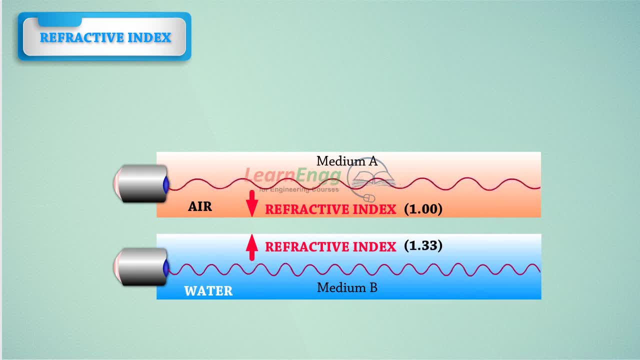 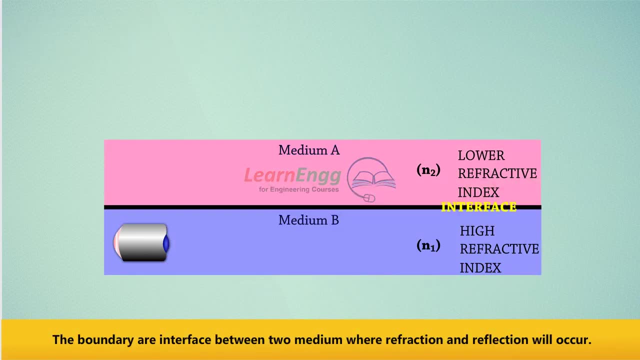 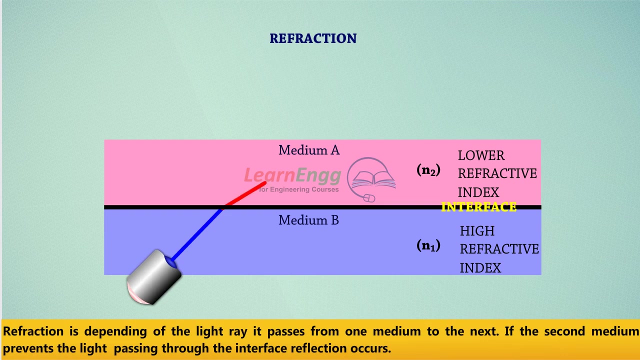 Air ray propagating through water will travel a slower speed than Air, The boundary or interface between two medium where refraction and reflection will occur. Refraction is depending of the light ray. it passes from one medium to the next. Root is the part of the light princess, like the light and 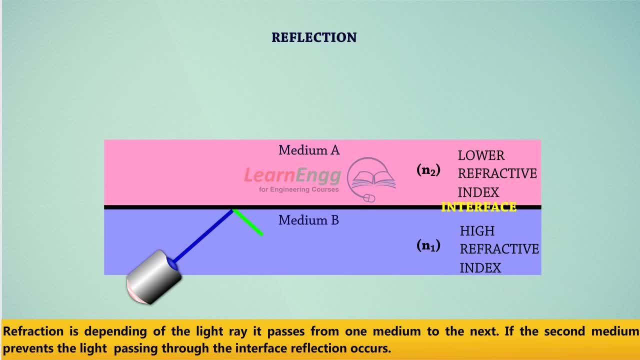 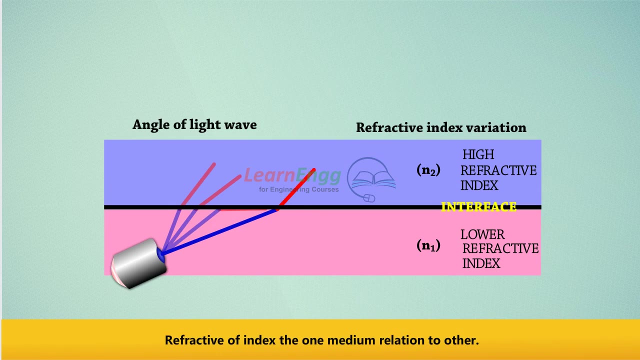 If the second medium prevents light from passing through the interface, reflection occurs. Two facts must be considered. Determine the degree of refraction or reflection: The angle of light, wave straights. the interface Refractive of index the one medium relation to the other. 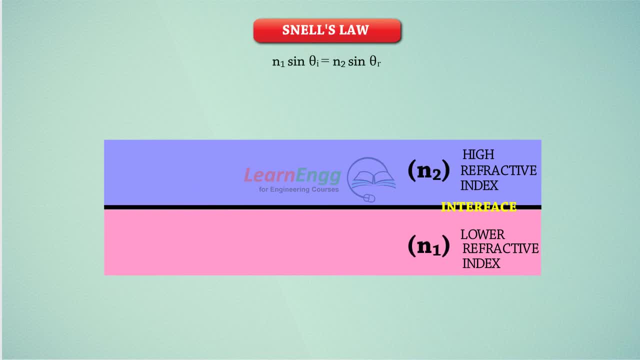 Snell's law is used to determine the angle of refraction between two mediums. Imaginary line is perpendicular to the interface. This line refer to as normal. A light ray is traveling straight into the new medium for long- the normal. It change speed but not change direction. 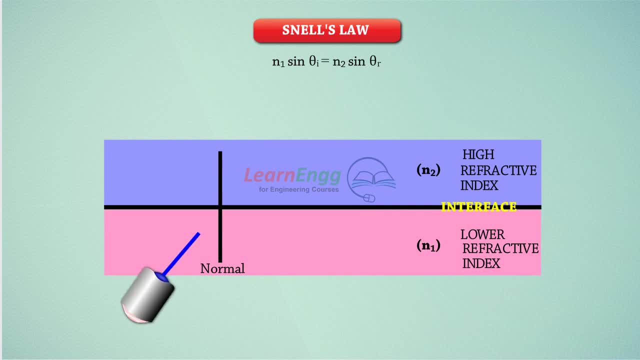 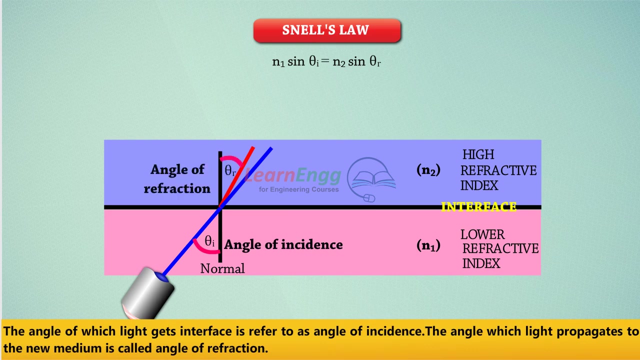 However, when light gets certain angle, it change in light speed and it cross the beam to change direction slightly and propagate to the second medium or different angle. The angle of which light hits interface Is refer to as the angle of incidence. The angle which light propagates to the new medium is called the angle of refraction. 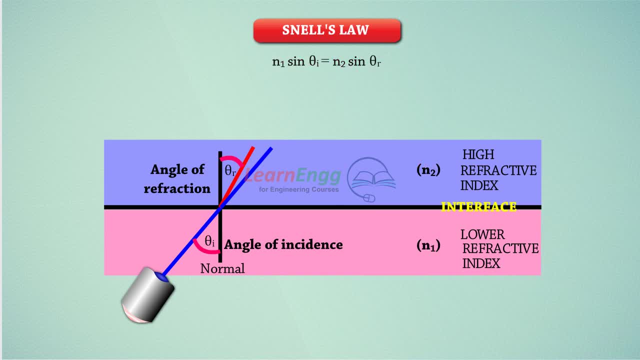 By placing the non-values in the Snell's formula, the degree of refraction can be determined. Snell's law states: the refractive index of the second medium is greater than first, But the angle of refraction is smaller than the angle of incidence. 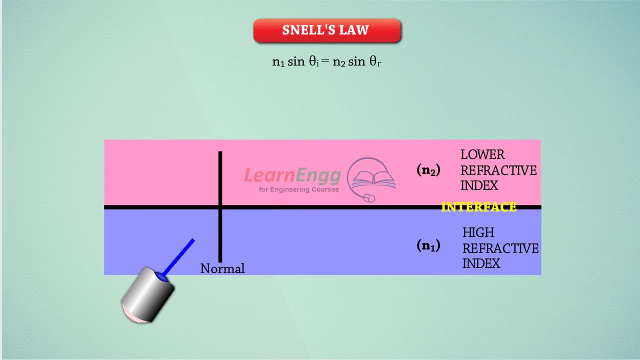 Conversely, the refractive index of the second medium is smaller than first. The angle of refraction is smaller than the angle of incidence. This is the principle. their neighbor like to travel. fiber optic stand, But the angle of refraction is higher than first. 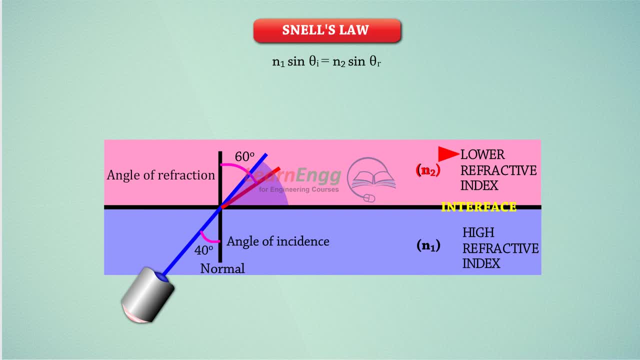 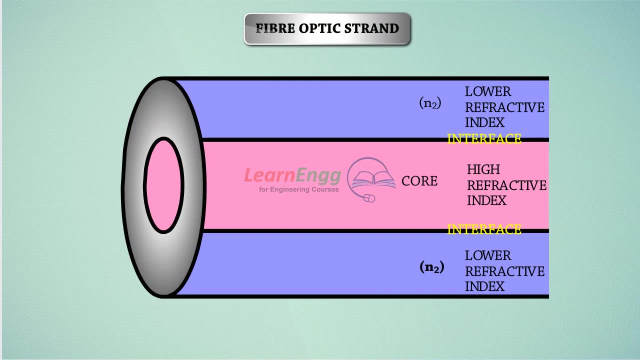 The angle of refraction is greater than the angle of incidence. This is the principle their neighbor like to travel. fiber optic stand Core have higher refractive index than the surrounding cladding. The light ray from the core will increase in speed in cladding which has lower refractive. 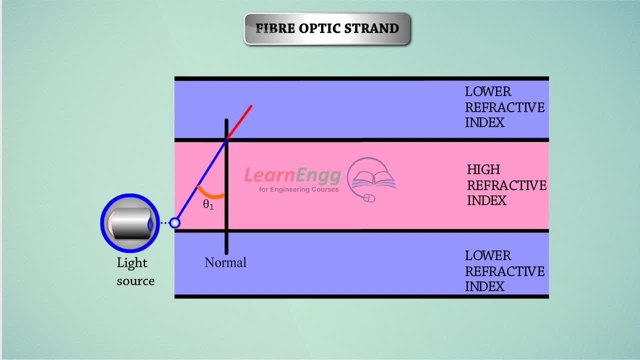 index. Notice: if the angle of incidence become greater, the angle of refraction approach the boundary or interface. If the angle of incidence is such refract lightweight travel long boundary between core and cladding- It is known as critical angle. If the angle of incidence is greater than the critical angle, the light will be reflected with no refraction. 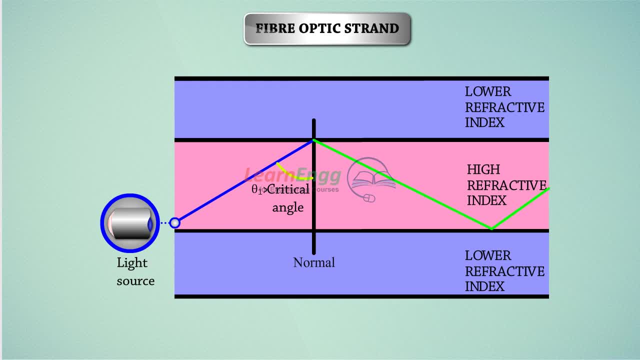 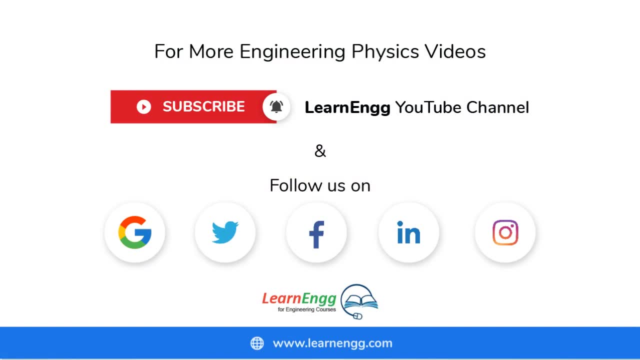 This is what known as total internal reflection Social media.